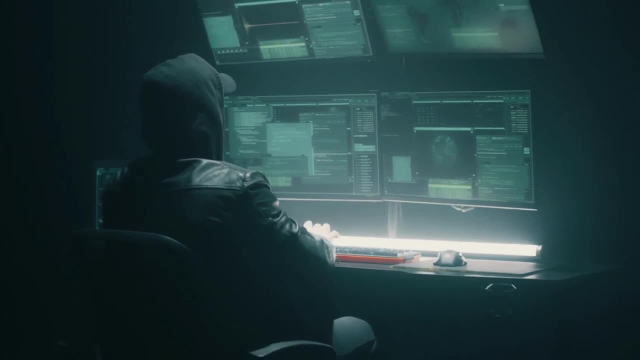 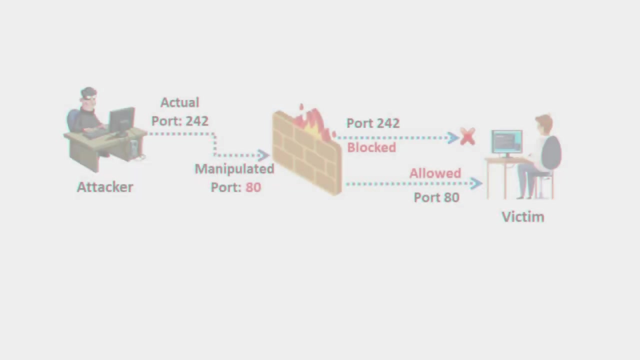 security systems. Picture this: you're an attacker aiming to slip past the watchful eyes of IDs and firewalls. Enter: source port manipulation, a tactic that involves playing with port numbers to outsmart the defenses. The trick lies in manipulating the source port numbers, swapping them with common port numbers. 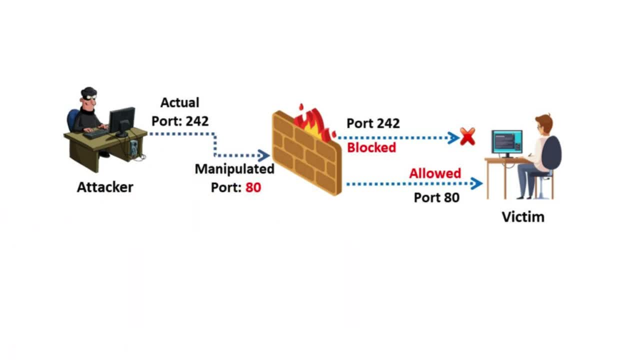 like HTTP, DNS or FTP, all while taking advantage of the blind trust in these well-known ports. Ever wondered how an administrator configures a firewall to allow traffic from those trusted ports? Think HTTP, think DNS- the usual suspects. But here's where the vulnerability creeps in. 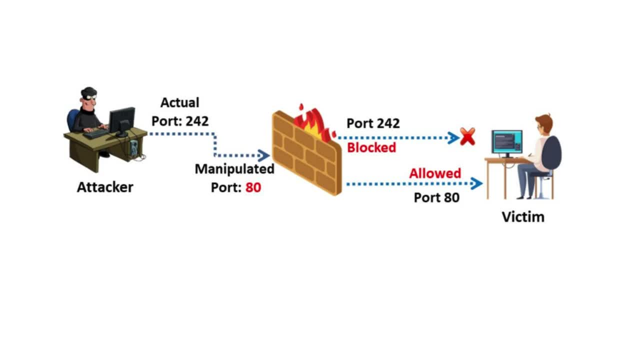 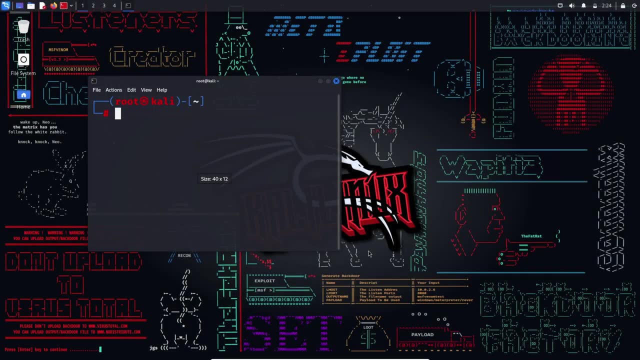 By blindly trusting these source port numbers, the firewall unwittingly opens the door to incoming traffic from attackers masquerading under the guise of common ports. In Django 4.1, two governments take over but never look back. whatnot the car around the colored fPop? 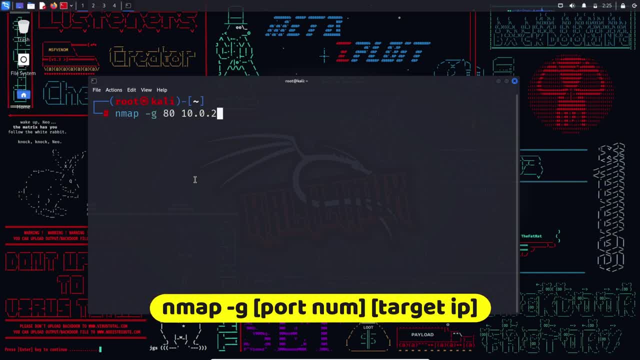 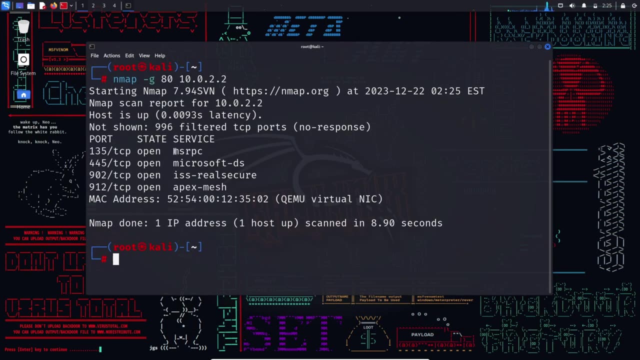 And in a Formula 1, you practically won't be standing somewhere else. upprove: The attaacker, armed with cunning tactics, can execute a maneuver like by typing nmap, target ip. Nmap, a powerful network scanning tool, is invoked with the g option, followed by the common port number 80 and the target's IP address. 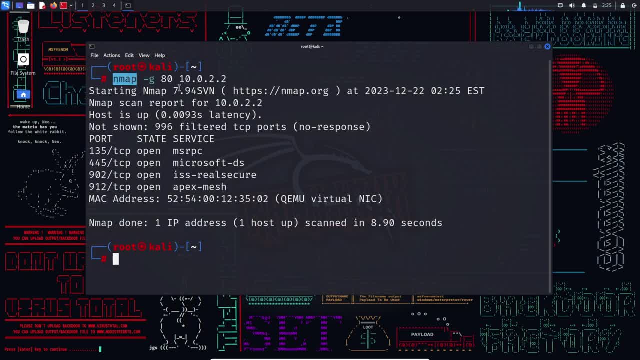 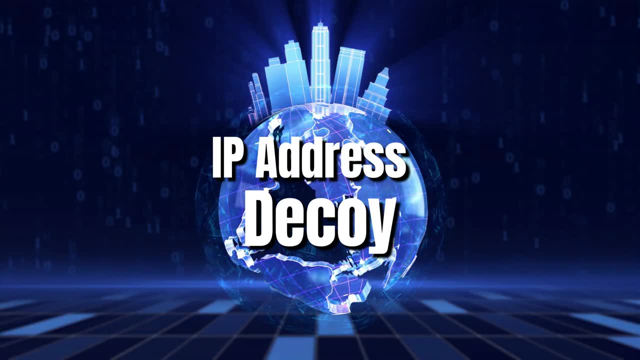 form, Nmap becomes the key to the kingdom, allowing the attacker to effortlessly tweak the original port number, slipping through the IDs and firewall undetected IP address decoy. Now let's uncover another fascinating technique in our quest to outsmart IDs and firewalls. 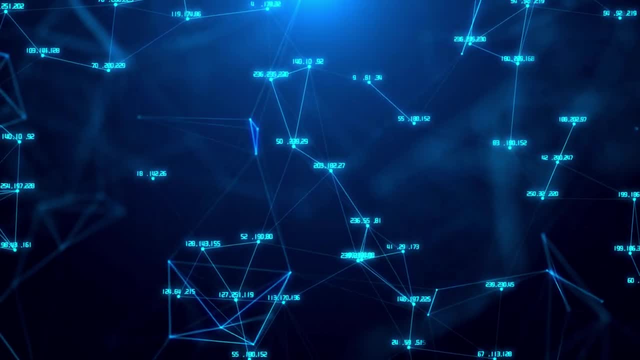 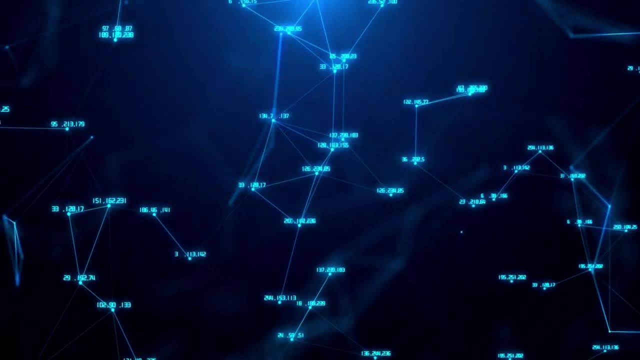 the IP address decoy. Imagine a digital ballet where the stage is crowded with decoys, making it near impossible for security mechanisms to distinguish the true performer from the ensemble. The IP address decoy technique revolves around creating a smokescreen of IP addresses. 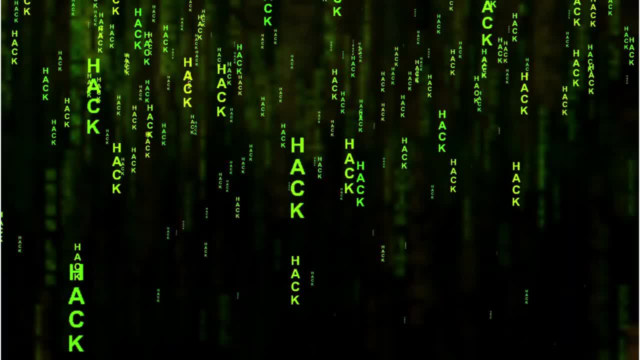 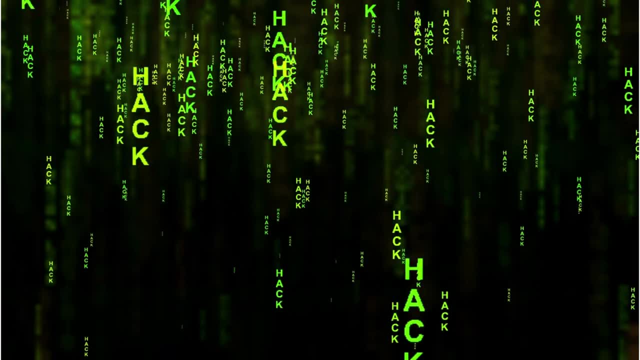 both manually specified and randomly generated. to cloak the true source of a scan. This confuses the IDs and firewalls, leaving them puzzled about which IP address is actually probing the network and which ones are mere decoys. Enter Nmap, the Swiss army knife of network scanning equipped. 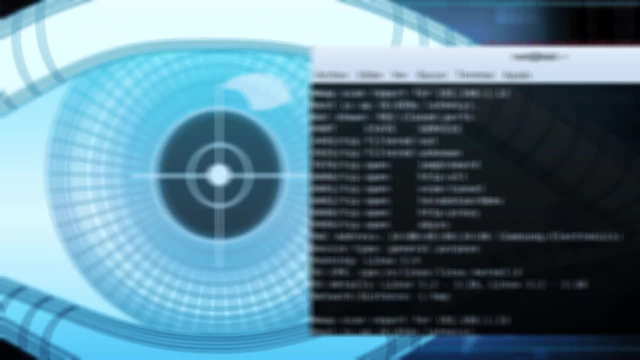 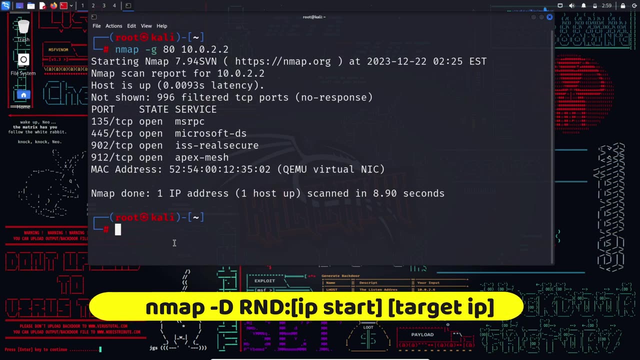 with a built-in decoy scan function. Let's explore two intriguing methods. The first one is random decoys. By typing nmap, d, rnd 10, target In this command, Nmap crafts a decoy scan with a random number of. 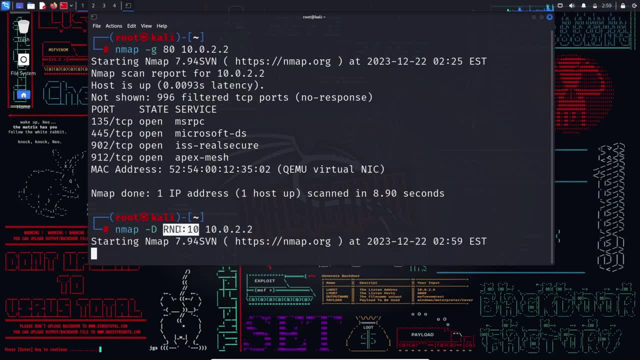 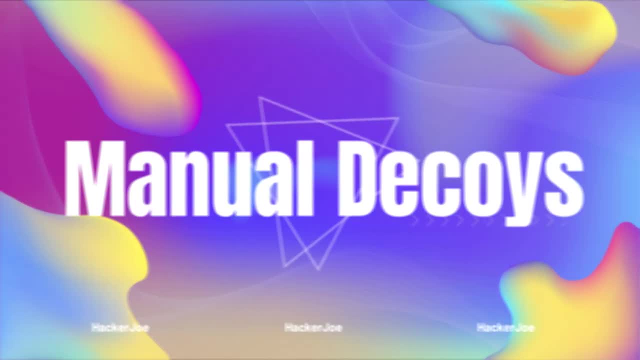 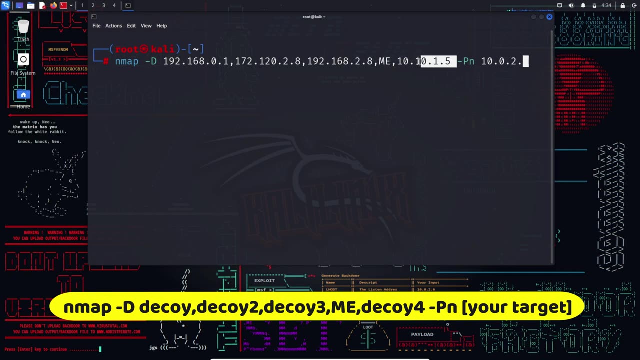 decoys, strategically positioning the real IP address amidst the decoy IPs. Picture a digital shell game that keeps the security mechanisms guessing. The second is manual decoys By typing nmap d, decoyl, decoy2, decoy3, me, decoy4- your target Using this command. 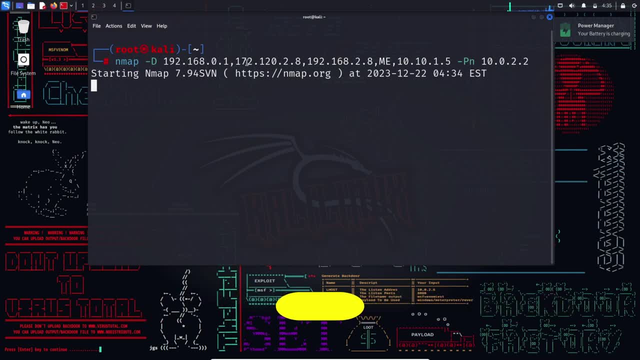 you can manually specify the IP addresses of the decoys to scan the victim's network. Here you have to separate each decoy IP with a comma, and you can optionally use the me command to position your real IP in the decoy list If you place me in the second position of the command. 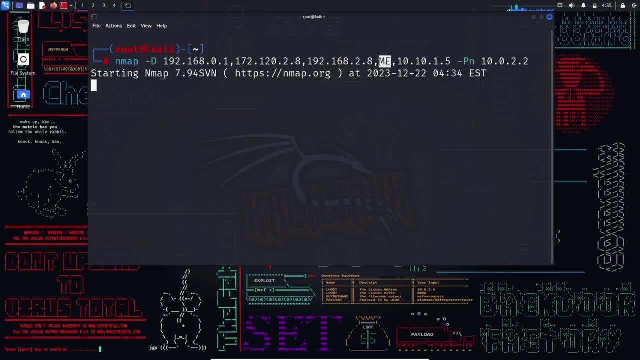 your real IP will be positioned at the second position accordingly. This is an optional command and if you do not mention a me in your scan command, then Nmap will automatically place your real IP in any random position. For example, assume that 10 0- 2.15 is the real source IP in. 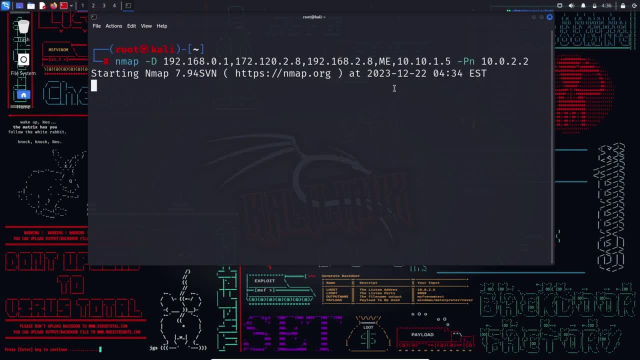 10 0, 2.2 is the target IP address to be scanned. These decoys can be generated in both initial ping scans, such as ICMP, SYN, ACK, etc. and during the actual port scanning phase. IP address decoy is. 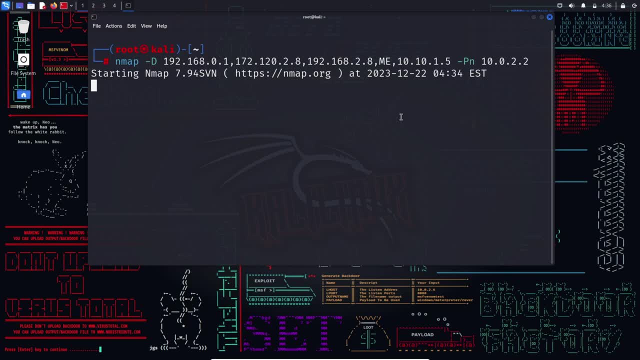 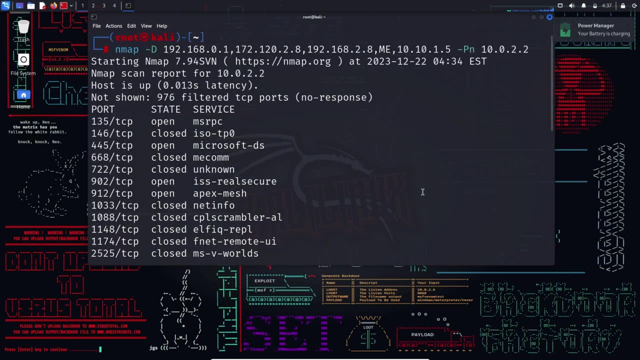 a useful technique for hiding your IP address. However, it will not be successful if the target employs active mechanisms such as router path tracing, response dropping, etc. Moreover, using many decoys can slow down the scanning process and affect the accuracy of the scan. 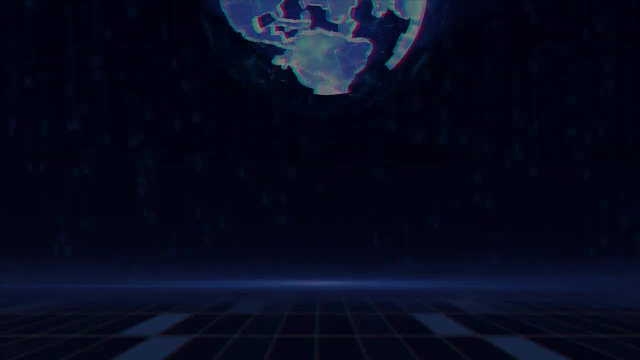 The next is nmap, d decoy2, decoy3, me, decoy4- your target IP address to be scanned If the target employs active mechanisms such as router path tracing, response dropping, etc. The next is IP address spoofing. Now let's unravel the clandestine art of IP address spoofing. 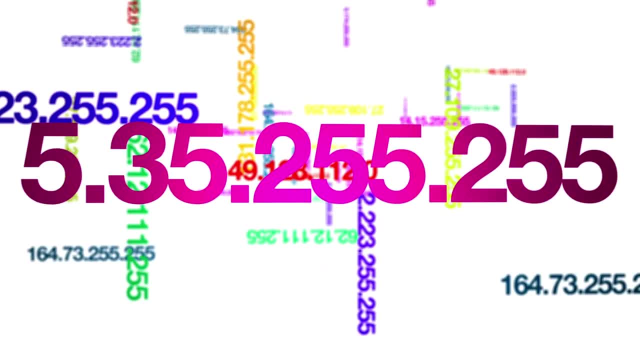 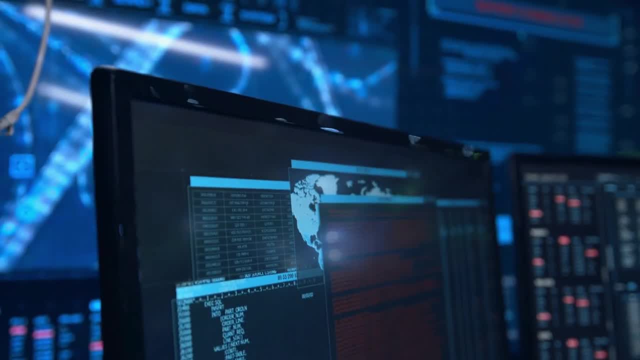 a technique that turns the tables on firewalls and IDs, allowing attackers to slip through the cracks. undetected Picture this: most firewalls stand guard by filtering packets based on the source IP address. They scrutinize incoming packets, trying to discern friend from foe. 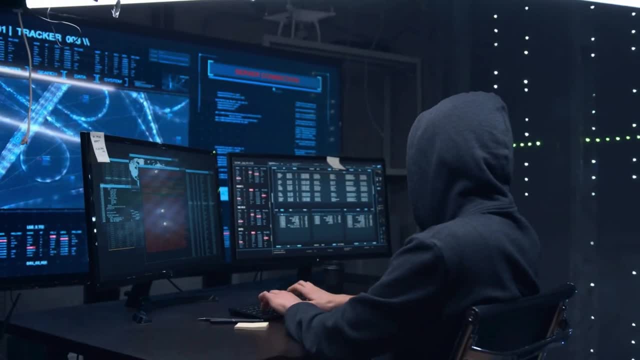 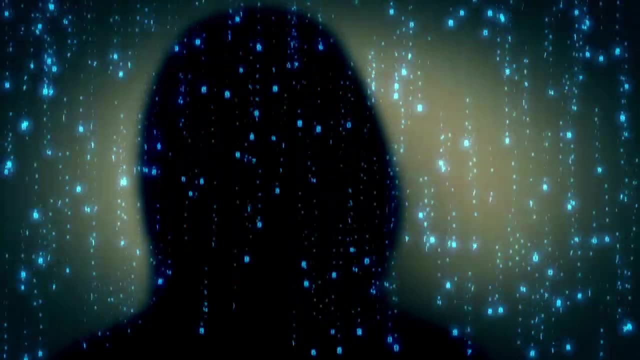 But here's where the game gets interesting. enter the IP address spoofing technique, a digital hijacking maneuver that puts attackers in the shadows. IP address spoofing involves an attacker masquerading as a legitimate host. by altering packet headers, The attacker. 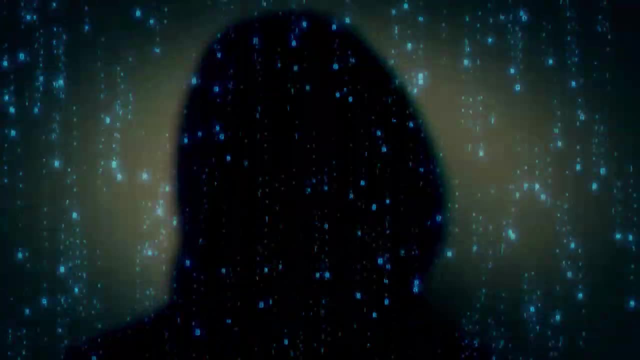 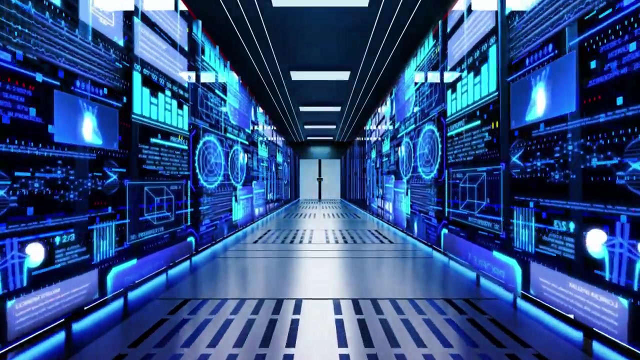 like a cunning puppeteer, sends request packets to a target machine, making it appear as if they're coming from a trustworthy source. However, the reality is quite different. these packets are crafted in the lair of the attacker with their true IP address cleverly concealed. 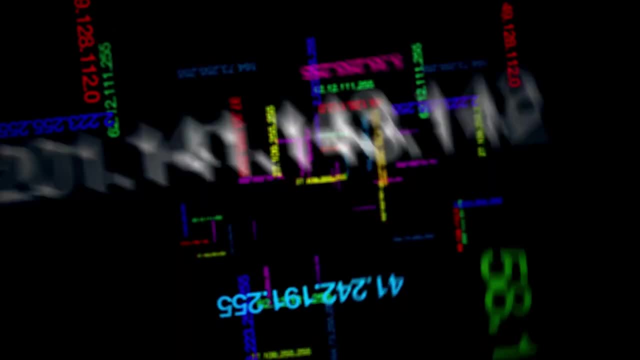 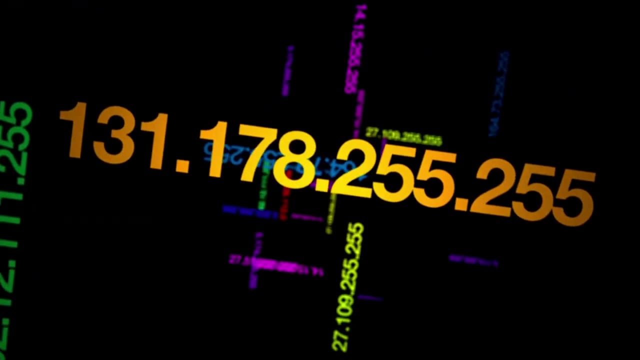 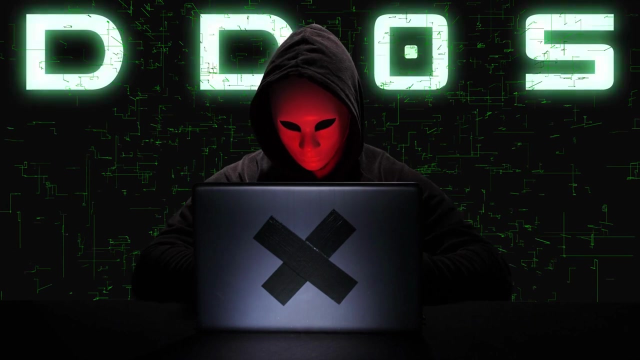 When the victim, unsuspecting, responds to the apparent legitimate address, it's actually replying to the spoofed address, not the attacker's real one. It's a digital shell game where the illusion of legitimacy is shattered upon closer inspection. Attackers often wield IP address spoofing as a weapon for DOS attacks. Imagine this scenario. 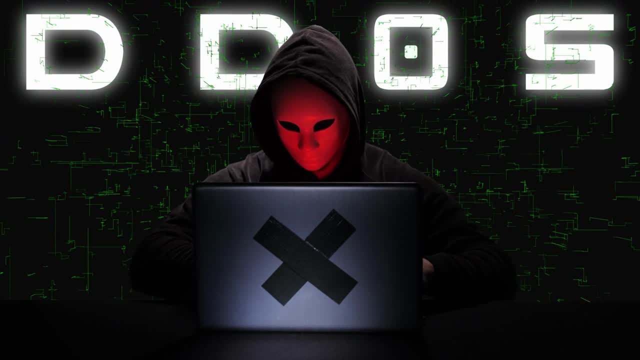 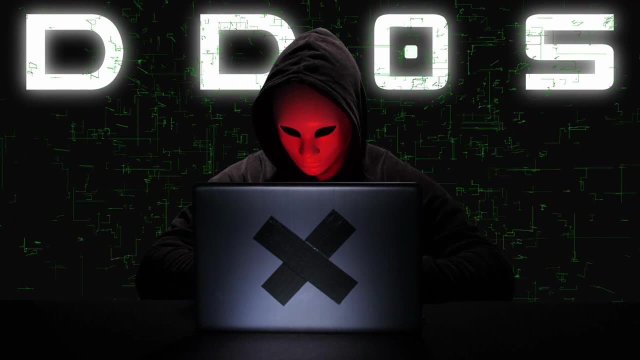 the attacker sends a connection request to the target host and the target dutifully responds to the spoofed IP address. If the attacker spoofs a non-existent address, the target replies to a non-existent system, leading to a waiting game until the session times out. The result: The 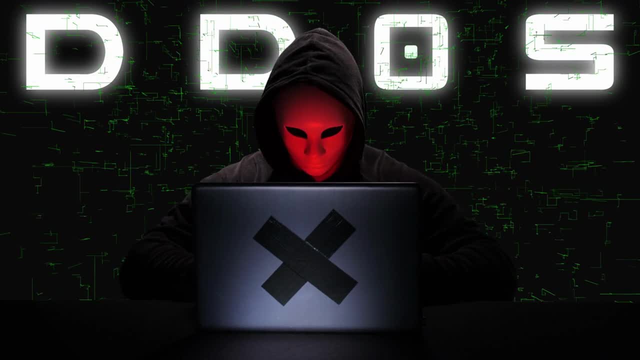 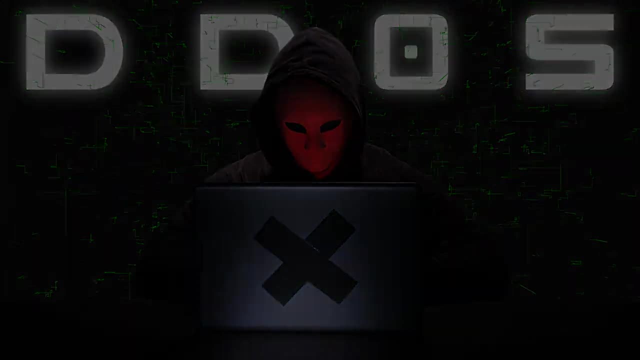 target unwittingly consumes a significant chunk of its resources. all under the puppet master's control. And remember that you will not be able to complete the three-way handshake and open a successful TCP connection with spoofed IP addresses- IP spoofing using hping3 with a. 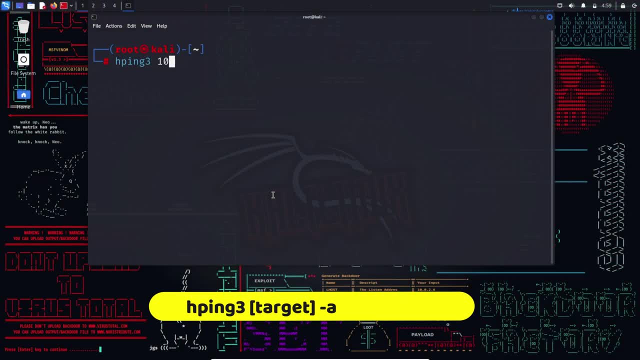 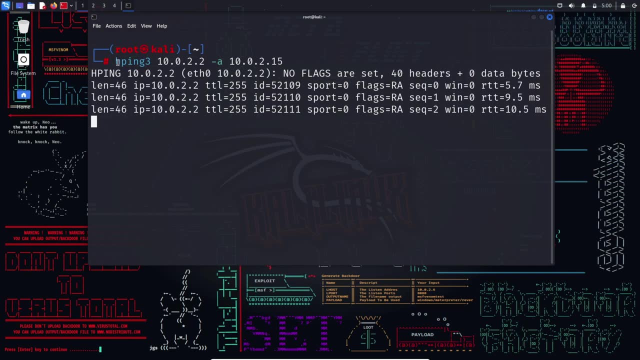 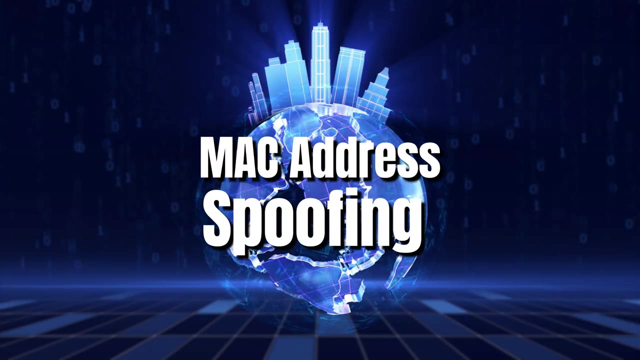 simple command. like hping3, your target a IP address, You can use hping3 to perform IP spoofing. The above command helps you to send arbitrary TCP IP packets to network hosts- NACK Address Spoofing. As we delve deeper into the 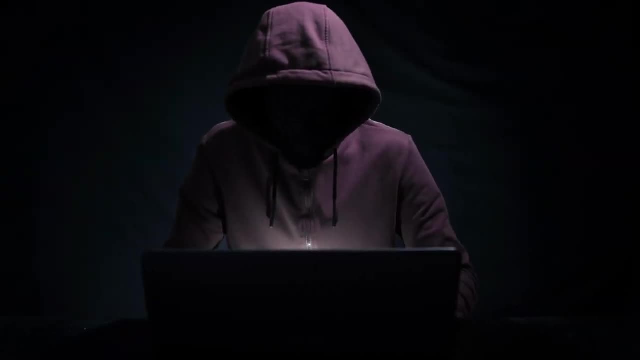 shadows of cybersecurity. our final stop is a technique that pulls attackers even further away from prying into the cyber security of the attacker's network. This is a technique that can be used to prevent attackers from spoofing. Imagine it as a digital mask allowing cyber. 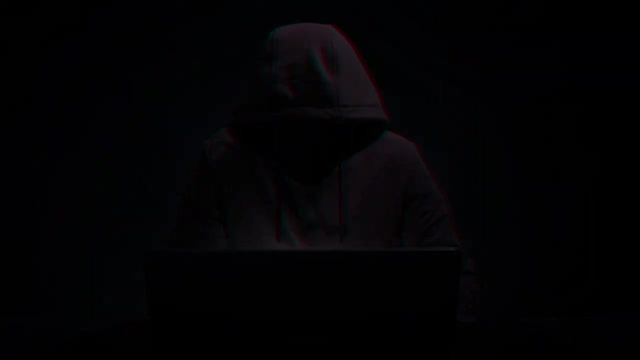 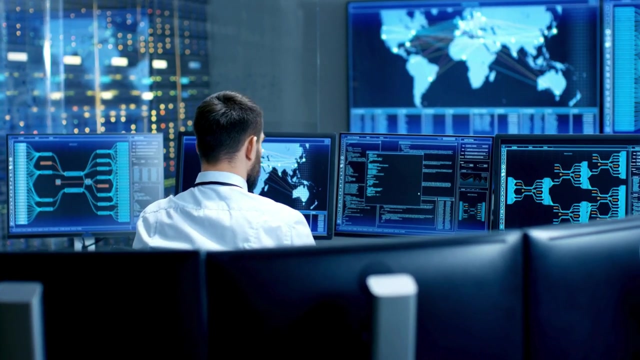 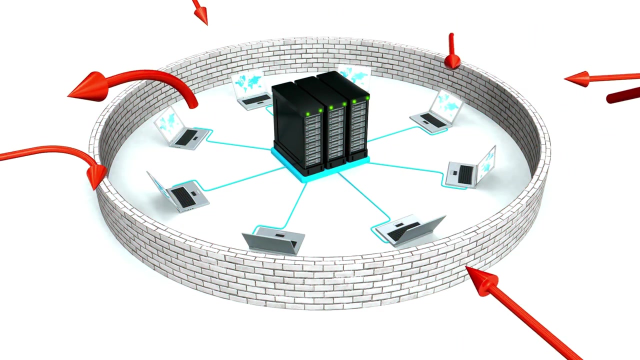 intruders to dance undetected within the intricate realms of network firewalls. Network firewalls ever watchful: filter packets based on the source media access control address. They meticulously examine these addresses in packet headers, distinguishing between friend and foe. But where there's scrutiny, there's also evasion, and attackers leverage MAC spoofing to 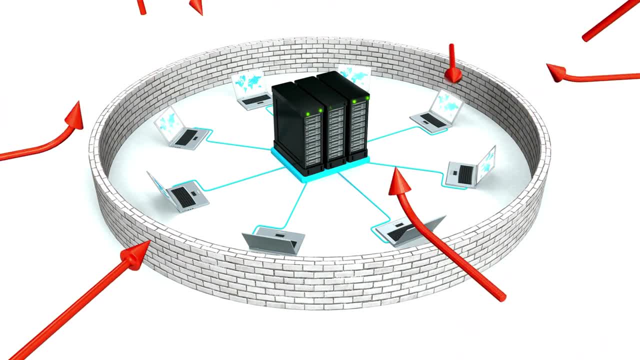 slip through undetected. Firewalls often employ MAC filtering rules to allow or restrict traffic based on specific networks. If you have a network that has a network that has a network that is spoofing, you can use the MAC spoofing technique To thwart these restrictions. 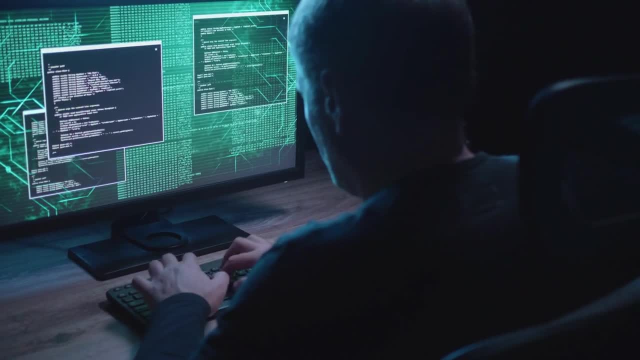 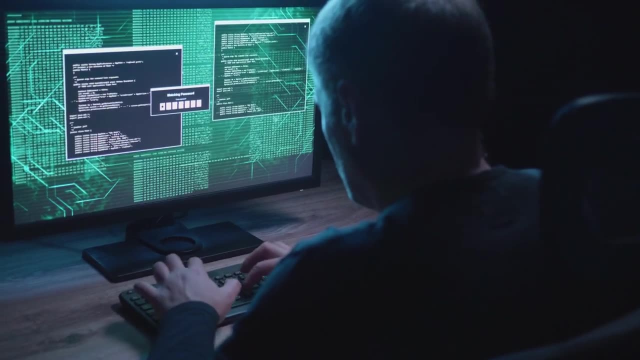 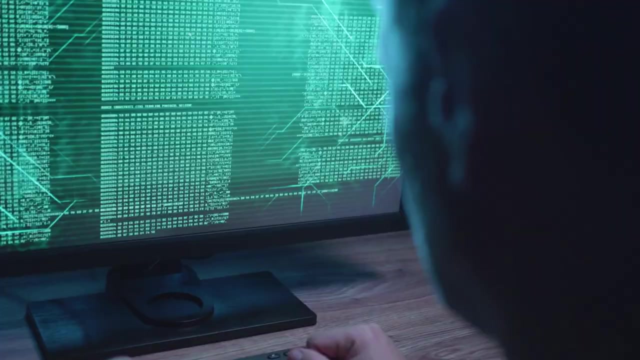 attackers adopt MAC spoofing techniques, crafting fake MAC addresses to pose as legitimate users and explore the hosts nestled behind the firewalls' defenses. The MAC address spoofing technique empowers attackers to send request packets to target machines or networks, all while pretending to be a bona fide host. To execute this maneuver, attackers turn to the infamous NMAP tool. a. 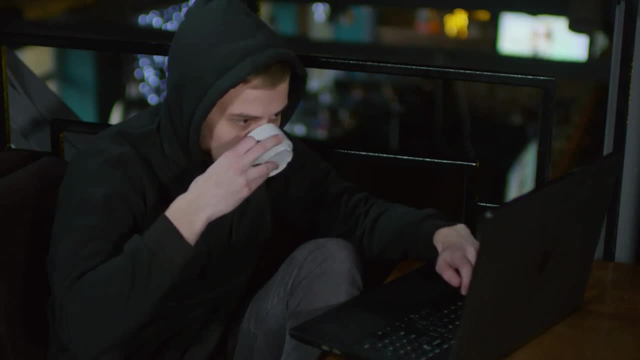